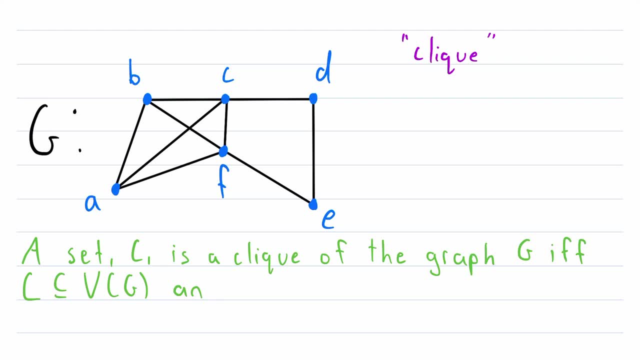 of the vertex set of G and every pair of distinct vertices in C is adjacent in G, And we can write that like this, Two vertices U and V being in the clique C, and this is a symbol for and and them. 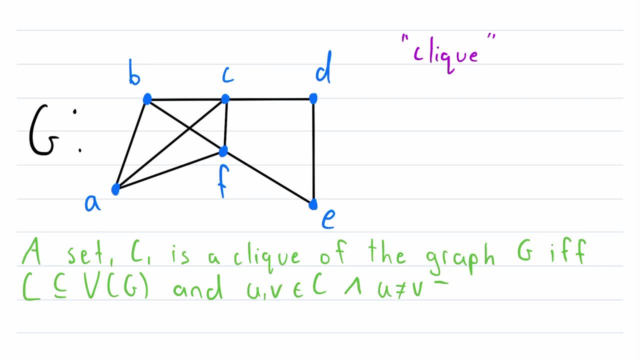 being distinct, so U is not equal to V. This implies that U and V are adjacent in G, which means that UV is an element Of the edge set of G, because there is an edge that joins them. So this is what a clique. 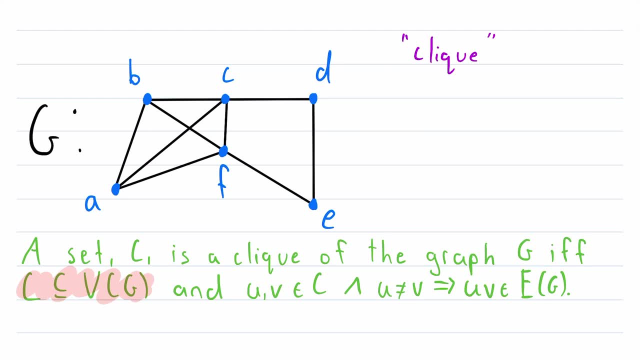 of a graph is. It's a subset of the vertex set such that all distinct vertices in the clique are joined by an edge. If you're familiar with induced subgraphs, you can also think of cliques like this: A set of vertices is a clique. if it's induced subgraph is a complete. 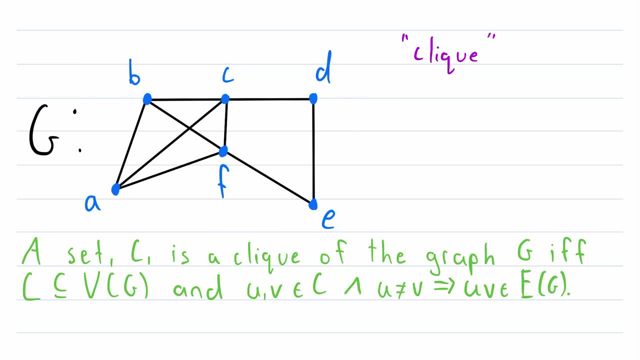 graph. So let's go ahead and look at a couple examples in our graph G. Take a moment and look at this graph. See if you can find a clique that has four vertices. Maybe pause the video and see if you can spot one. All right, maybe you found one, maybe. 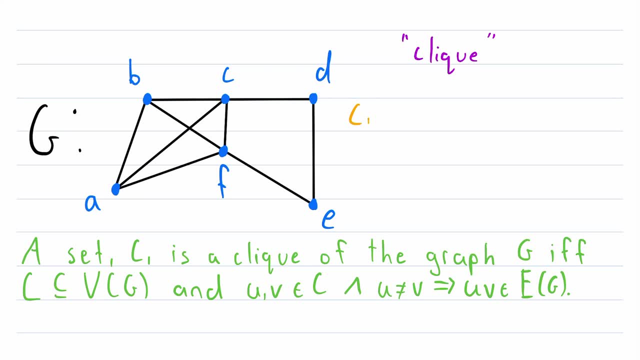 you didn't. Here's what I was looking at. Let's call this clique C1.. This clique is equal to the set containing the vertices A, B, C and F. So this clique, this C1, this is a clique of the graph G. Why is it a clique? 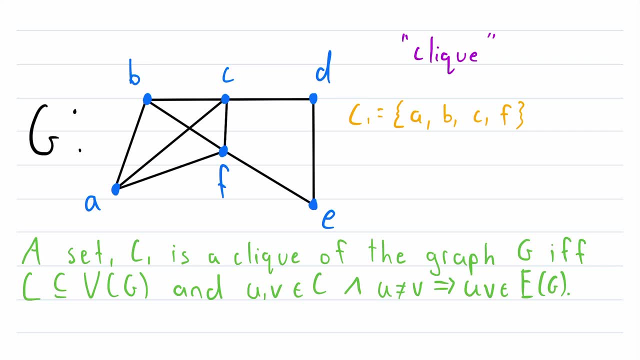 Because it is a subset of the vertex set of G. We can see that clearly, every vertex in C1 is a vertex of the graph G And then, secondly, every pair of distinct vertices in the set C1 is adjacent in G, For example the vertices A and F, A and F are adjacent in G, Another. 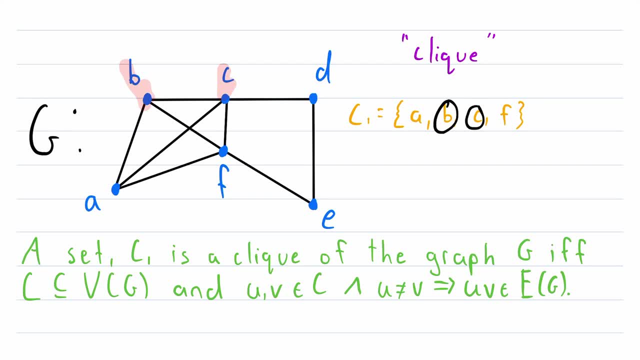 example, B and C. B and C are also adjacent in G. we could look at, let's say, B and F. B and F are also adjacent in G. So every pair of distinct vertices in C1 is adjacent in G. So it is a click And just to drive the point home further. 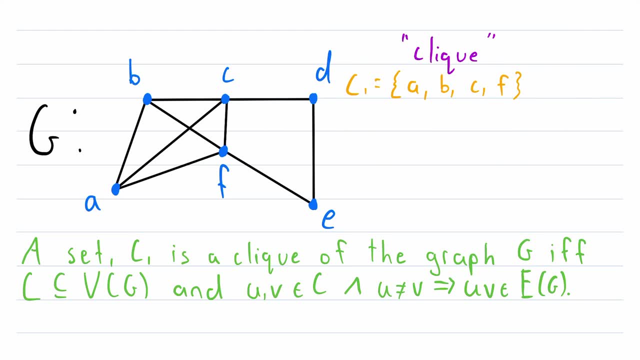 we could sketch the sub graph induced by this click And if you're not familiar with what that means, the sub graph induced by vertex set is just all of the vertices in the set. So B that's a little ugly. Let me write that B again if I could just hit this undo button really hard. 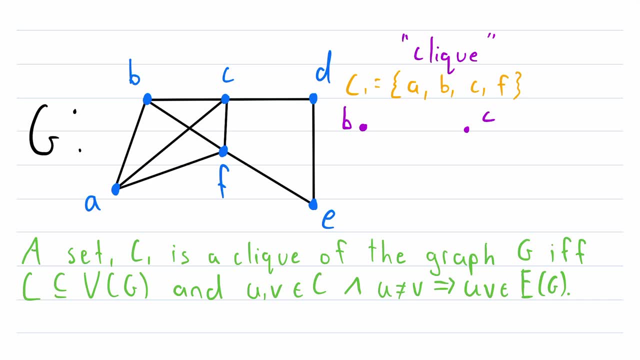 to hit vertex B, vertex C, vertex F and vertex A, so all the vertices in our set, as well as the edges that join those vertices in G. So in this case there's an edge joining B and C. there's an edge joining B and C. There's an edge joining B and C and so on And there's an phenomenal view of everything that's I can't explain. And it shows in the censored therapies that our h 1,, 2,, 4 and 5 have always shown. thatular device does not give you the suggestion. 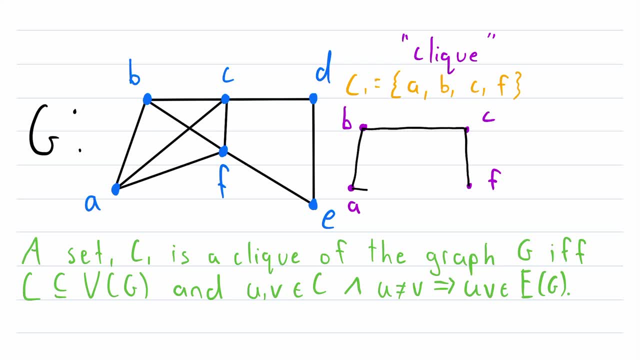 that others don't, And in that case these are just plain and normal. So hur cries their PCs, whether you see a per travail when I realized that it will take to them. and, of course, joining B and A: there's an edge. joining C and F: there's an edge, joining A and F. 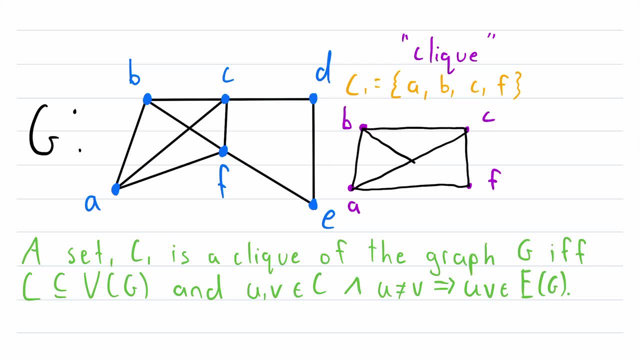 there's an edge joining A and C and there's an edge joining B and F. So again, this is the subgraph of G that is induced by this vertex set. It has all the vertices of our clique as well as the edges in G that join those vertices. 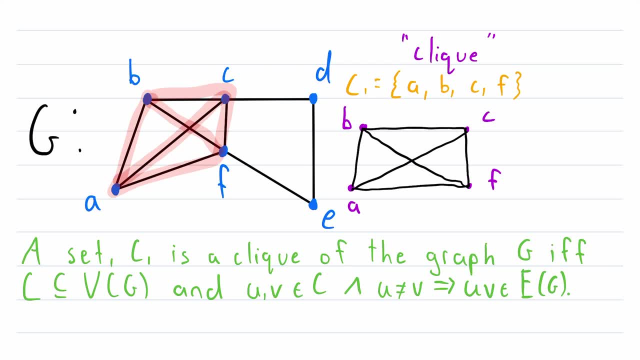 It's this piece of G right here and you can see that it is a complete graph And, by definition of a clique, that will always be the case. The subgraph induced by a clique is a complete graph. So that's well and good. Let's look at a non. 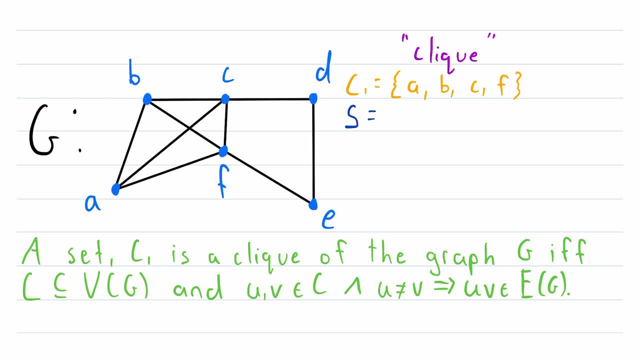 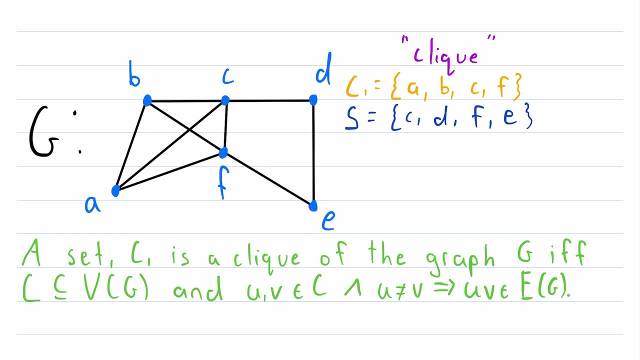 example. now We'll just call this vertex set S and let's say it includes C, D, F and E. This is not a clique. Although it is a subset of the vertex set of G, not every pair of distinct vertices in this set is adjacent. 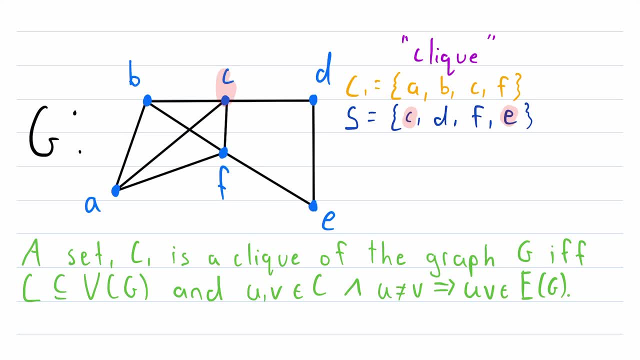 For example, the vertex C and the vertex E. we see that these two vertices are not adjacent in the graph, So this is not a clique. The subgraph induced by this vertex set is not a complete graph. For another example of a set that is a clique. 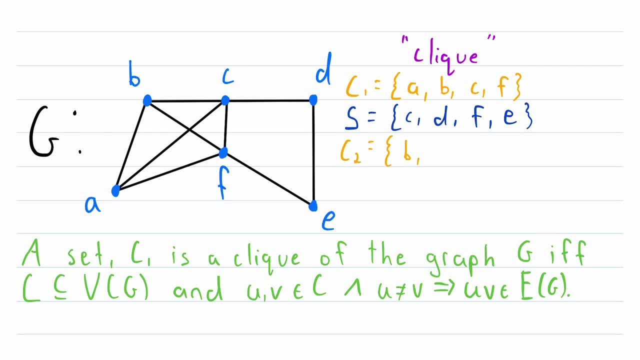 let's call this C2.. This set has the vertex B, the vertex C and the vertex F, And we can see just by looking over here that every pair of these three vertices is adjacent. B and C are adjacent, B and F are adjacent, and C and F are adjacent.